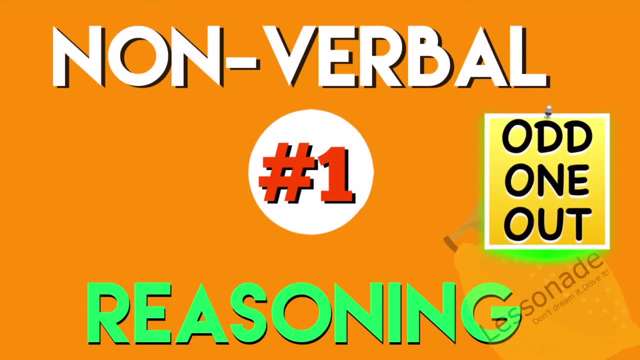 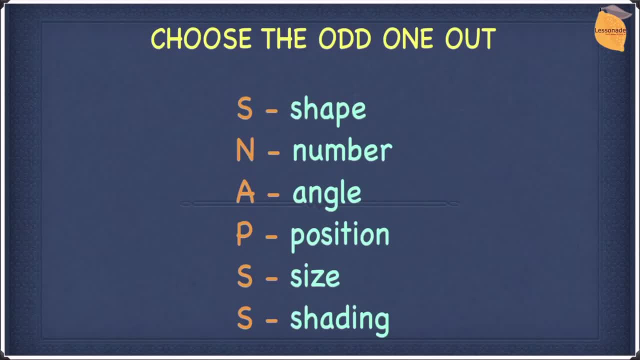 In this video you will learn non-verbal reasoning, type 1. Find the odd one out. Welcome to another video. If this is your first time here and you want to master 11 plus exam techniques to land in your dream grammar school, start right now by subscribing and clicking on. 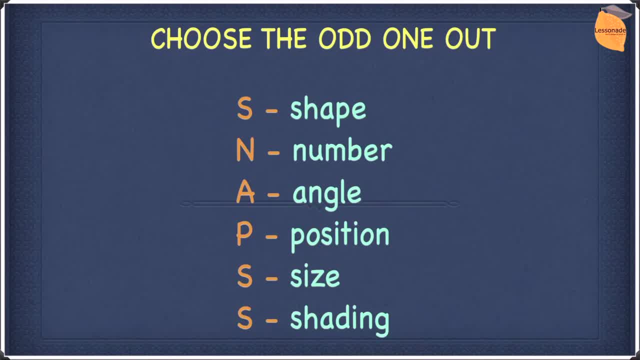 the bell so you don't miss anything. Before we start into these questions, let's first look at snaps. So snaps is S-N-A-P-S-S. S stands for shape. One shape might be different to the others. N stands for number. The number of shapes or the number of sides in a shape could be different. 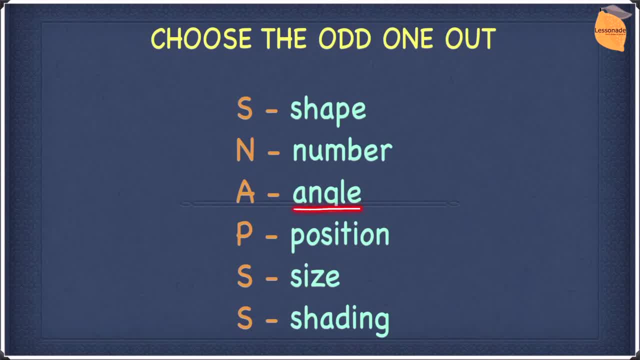 A stands for angle- The angle of a shape might be different- reflection or its rotation. P- the position of a shape might be different. S is size: The size of a shape could be different. And finally, S Is shading: The shading or a color of a shape could be different, Since we now know what snaps. 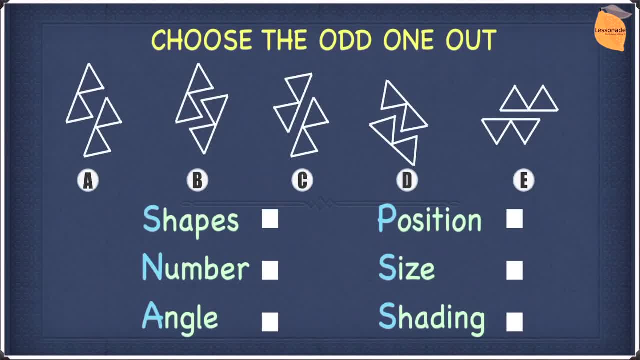 is. let's look at our first example. So let's look at this example. In this example, we have five options- A, B, C, D and E- and four of the options are related to each other, but one of them is: 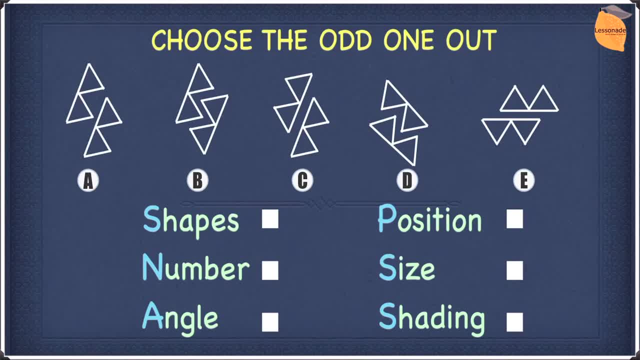 different. Our job is to find the different one, which will be the odd one out. So let's use snaps to find the answer. So snaps stands for shapes, number, angle, position, size and shading. Let's first use shapes. All of the options above have the. 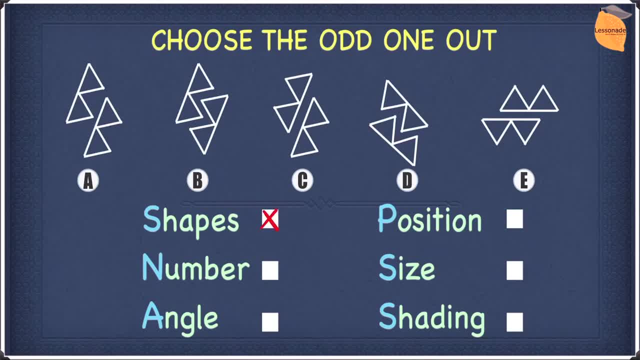 same shape, so we cannot use shapes. Let's move on to number. All of the options above have two shapes. This means we cannot use number either, So let's go on to angle. In terms of angle- option A, both of the shapes point in the same direction. In option B, they point in the opposite. 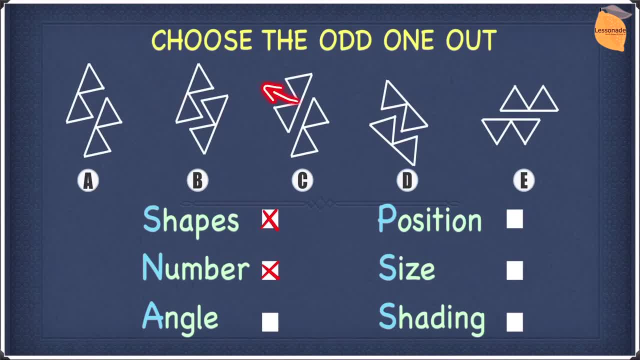 direction. In option C, they point in the opposite direction. In option D, they point in the opposite direction. In option C, they point in the opposite direction. In option C, they point in the opposite. and in option D, they once again point in the opposite direction. and finally in 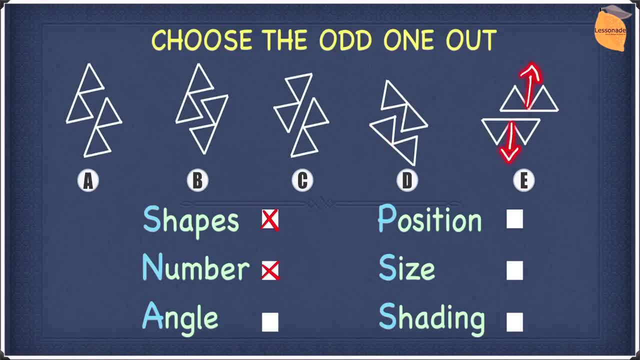 option E. they point in the opposite direction. This means our odd one out for this example is going to be A, because only in A we have both the shapes that point in the same direction. however, for the rest they all point in the opposite direction. So we can safely say our answer to this question is A, So I hope. 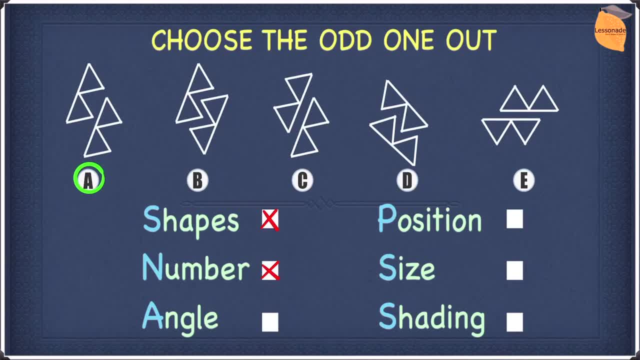 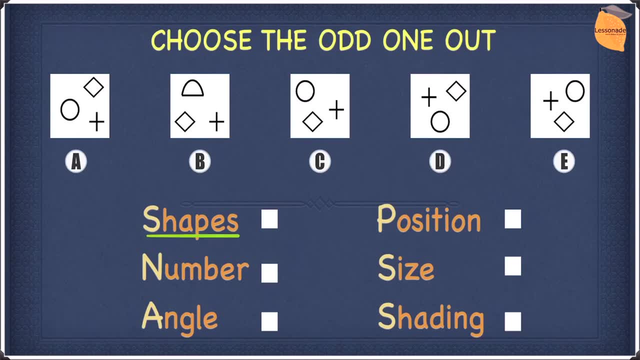 you guys understood everything so far. now let's go on to the next one. For this example, using snaps, we're going to first compare the shapes. So in all of the options above we can say that A, B, C, D and E- they all contain a plus. so B, C, D. 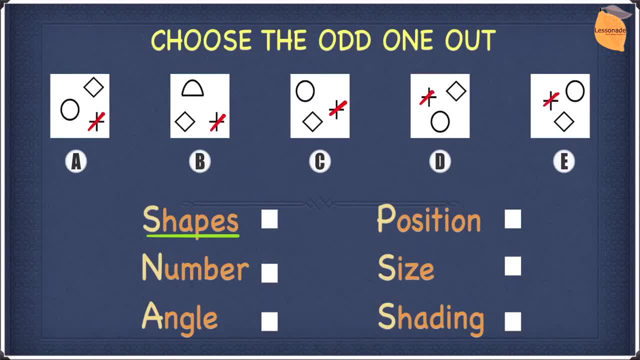 and E, and also they all contain a diamond: A contains one, B, C, D contains, and E contains a diamond as well. So all of them contain a diamond. A contains one, B, C, D contains, and E contains a diamond as well. So all of them. 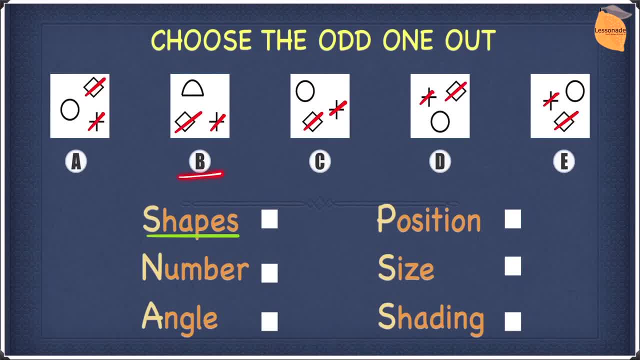 contain a diamond, but all of the options except for B, they all contain a circle. So A contains a circle, C contains one, D contains a circle and E contains a circle, But in B, however, instead of circle it has been replaced with a semicircle. So, since a semicircle is not a circle, this means our answer is: 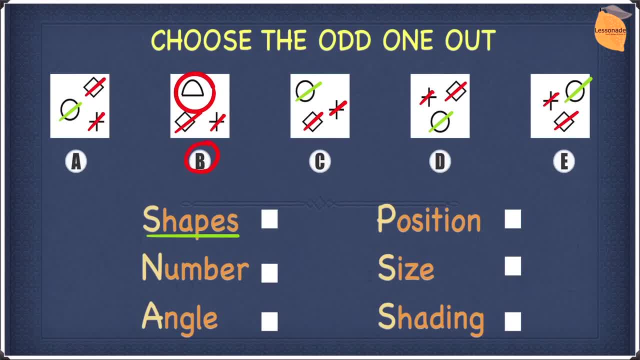 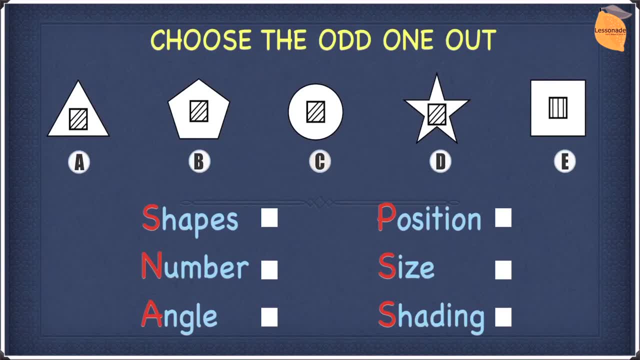 for this question is B, because B is the odd one out. So I hope you guys understood everything so far. now let's go on to the next one. Let's look at this example and let's use snaps to get our answer. So the first thing we have is shapes. So all of the options above. 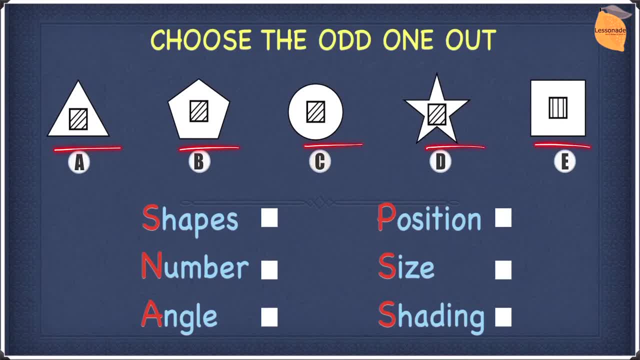 they have different shapes, which means shape does not work. So we can cross it off. Let's move on to numbers. All of the options above. they have two shapes: a smaller shape in the middle and a larger shape outside. So this means number doesn't work either. So let's look at angle. All of the 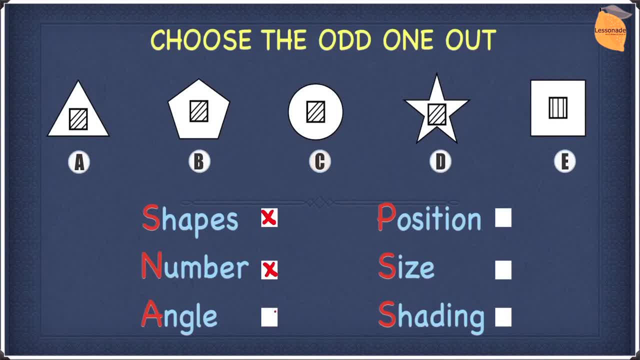 shapes above. they have different angles, so angle doesn't work in terms of position. the position of the shape is the same because if you look at the inner shape, it's always in the middle. so for a, b, c, d and e, the inner shape is always in the middle. so we cannot use this as an option to find the odd one out. so let's move on to